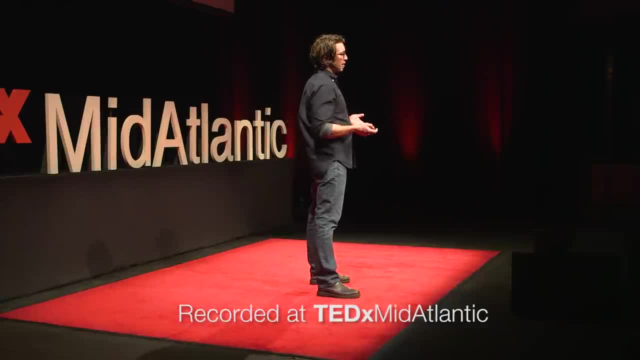 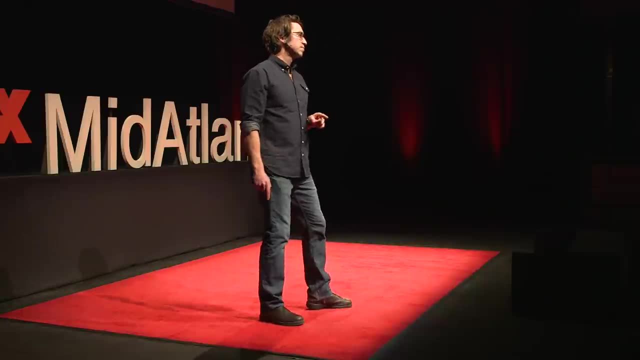 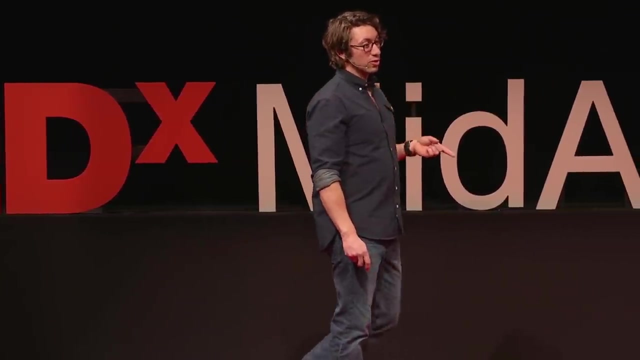 and I've never worked in PR. What I am is a psychological anthropologist, And what I study is the way that culture influences how we think, how we process information, how we make meaning of messages and how we formulate and come to decisions. And so, as a psychological 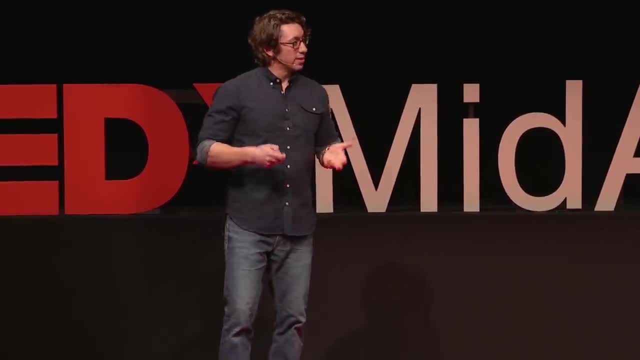 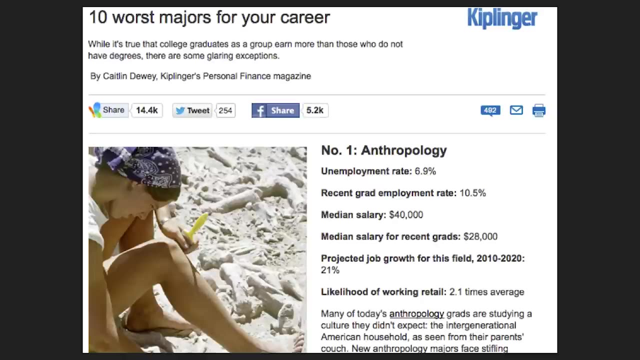 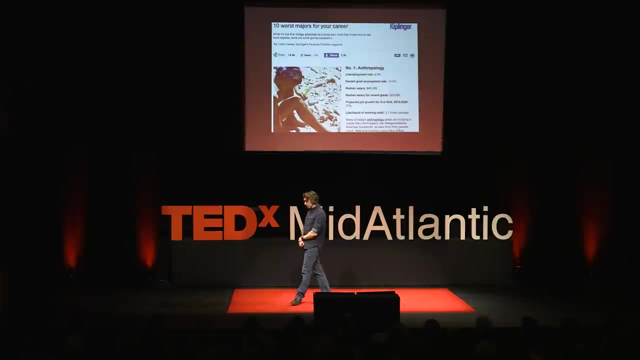 anthropologist. one of my goals here today is to convince you, is to show you, that this is not true, That we should not be actively dissuading our friends and colleagues from going into anthropology, and that, instead, studying culture and how people use it to think is an incredibly 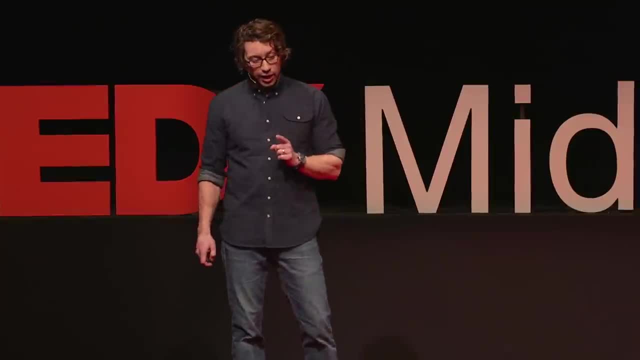 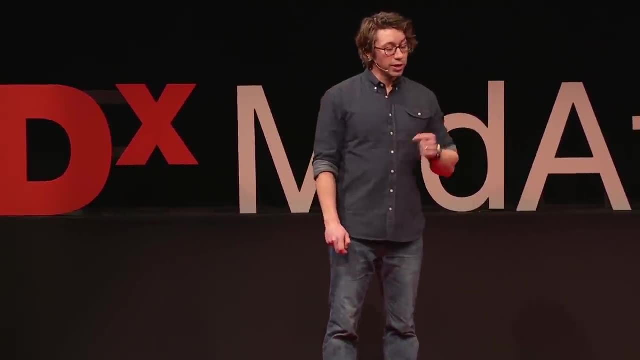 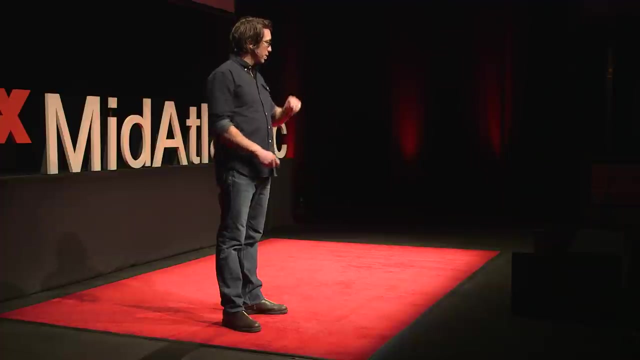 valuable tool in the real world and, for our purposes today, can be an incredibly important and effective thing in being a better communicator, And so, as an anthropologist working in communications, I study two different things. First of all, I study public thinking, Not public opinion, not the way that people answer. 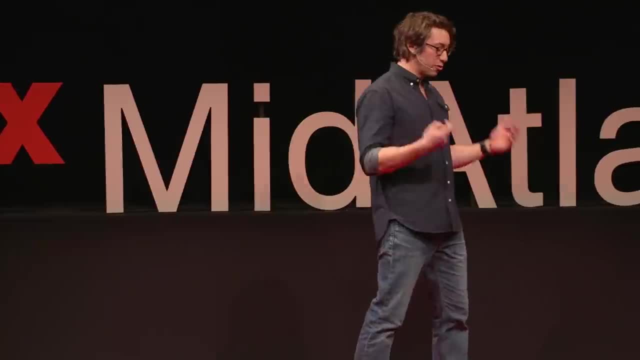 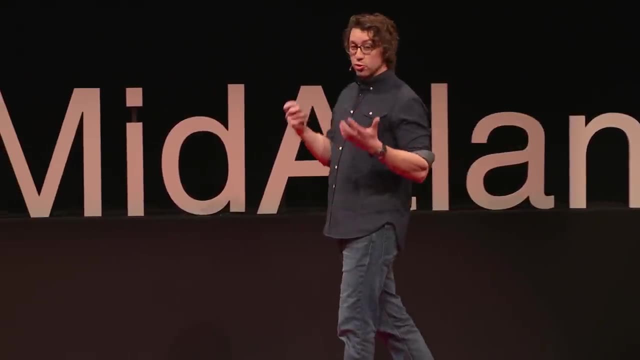 a couple of polling questions here or there conduct themselves in a few focus groups in Cleveland or Kansas City- I'm from Cleveland, I can make that joke, that's okay- But rather how people use culture in a deep and highly predictable way to think about complex social. 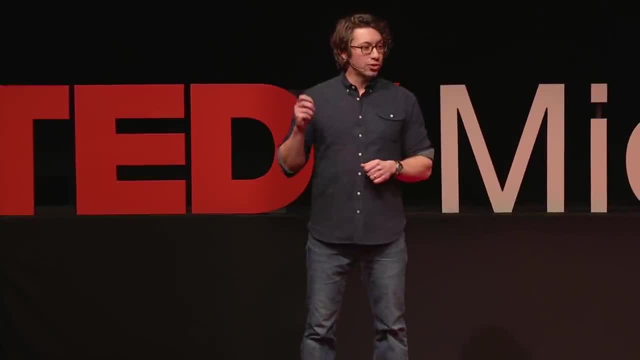 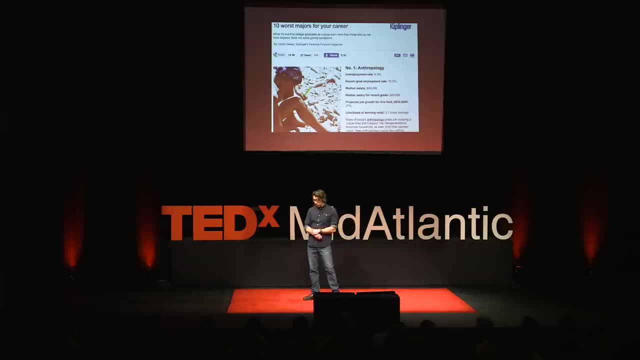 issues, Issues like education or mental health, immigration or aging, climate change or race and equity, And so I am really excited to talk to you about this kind of how culture helps us be more effective communicators. The other thing that I'm going to talk to you about is how 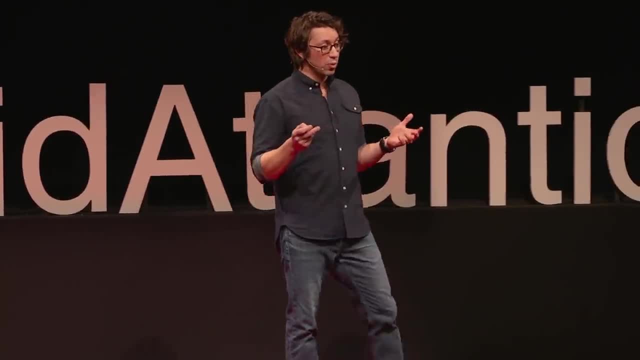 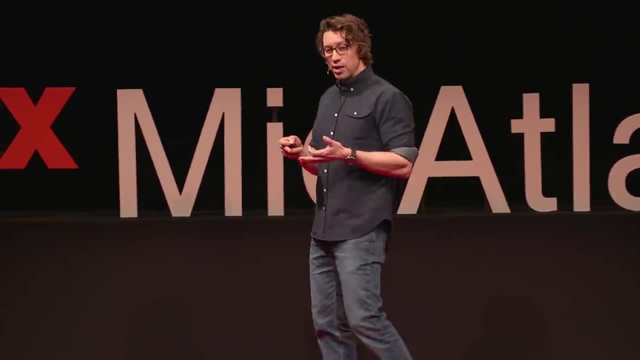 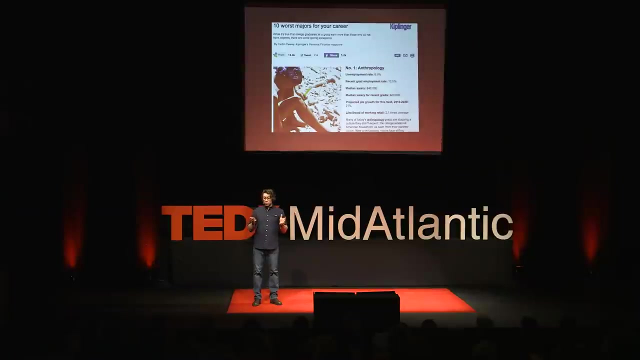 through the way that we present information, we can get people to open up and access dramatically different ways of thinking, of feeling and of acting about those social issues. And, in a nutshell, that is what framing is Now. variations in the way that we present information can lead people to dramatically 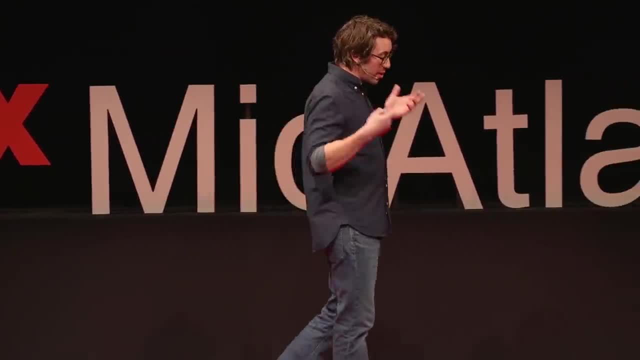 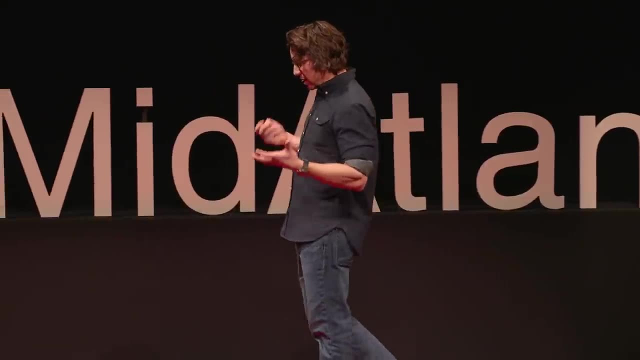 different perceptual and behavioral outcomes, And so I'm really really- why not really- excited to get the chance to geek out with you about framing today, And you all should know right from the beginning that geeking out about framing is pretty much my all-time. 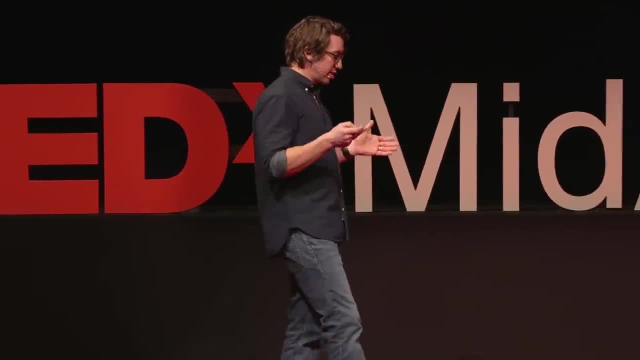 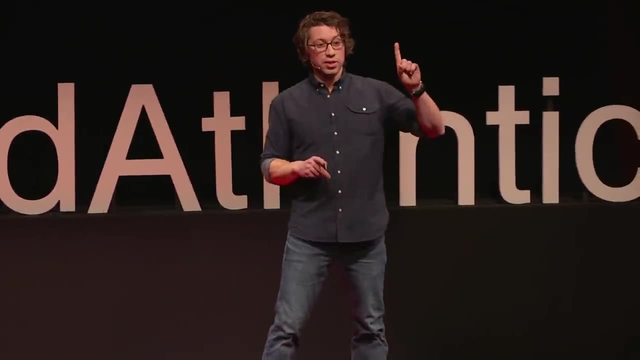 absolute favorite thing to do, which I realize is kind of pathetic and probably a little bit sad, but it does mean that at least one person in this room is going to have fun during this talk. That will be me. I will have fun. 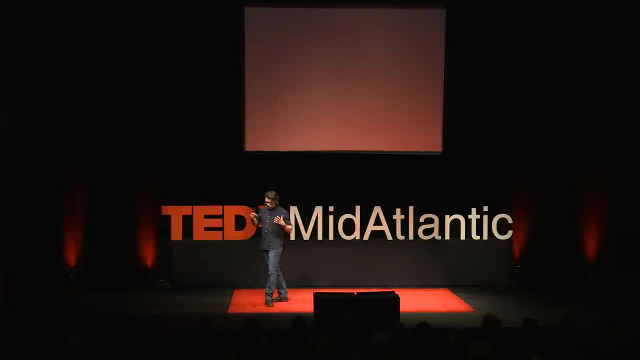 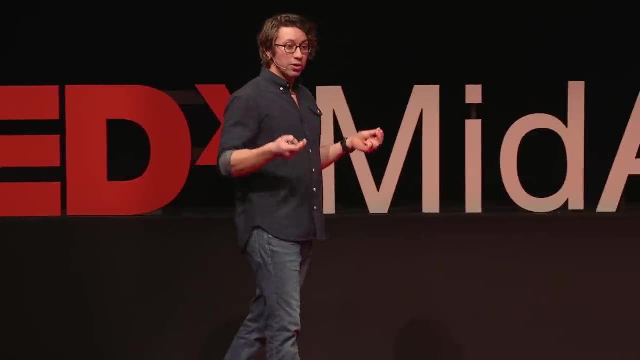 And so what I want to do today is to convince you, is to argue that, even though you do not think of yourselves all the time in this way and are not explicitly aware of it, you are all communicators And, as communicators, framing matters a great deal to you. So what I want 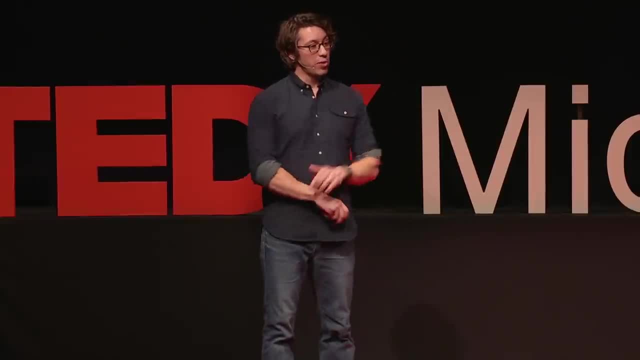 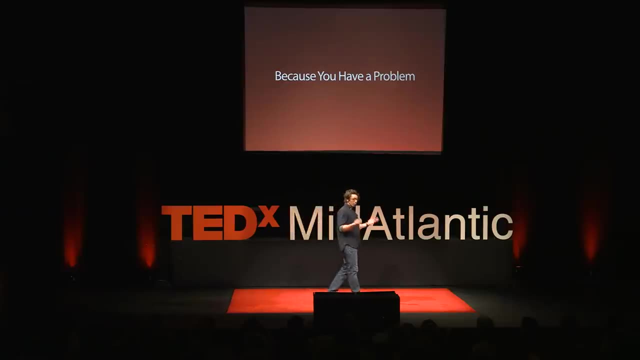 to do is give you two reasons why framing matters to you, and the first reason is, unfortunately, I'm in the position where I have to tell you that you all have a problem, and you should know there aren't 11 more steps after this. it's not that kind of a meeting, and 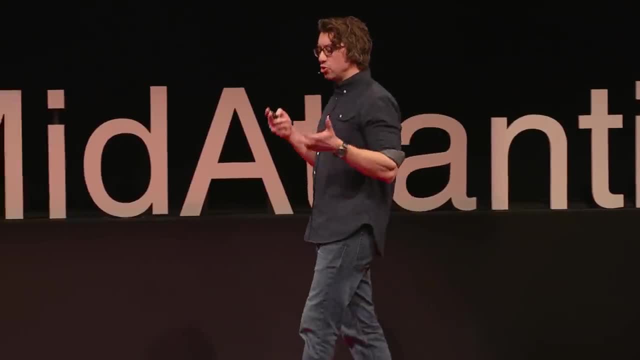 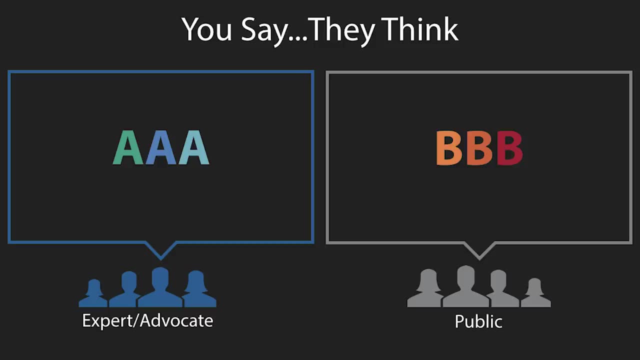 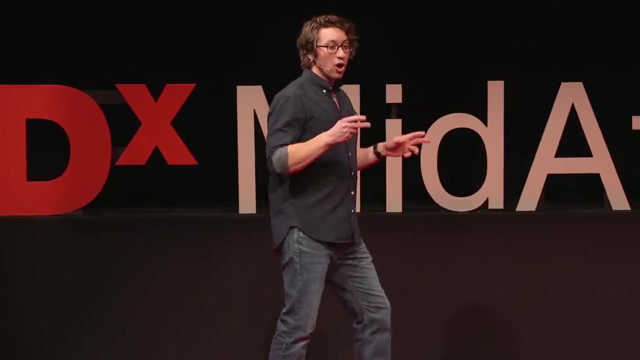 it's not that kind of a problem. what I mean is that you have a communications problem. you have a problem of perception, and the problem looks something like this: that you all have been in positions at one time or another where you think you have the most perfect, awesome slam-dunk- whatever sports metaphor you 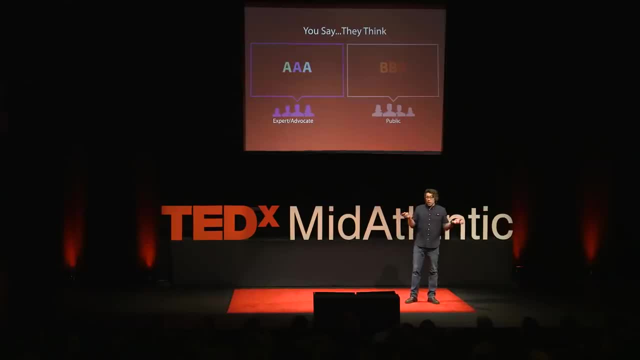 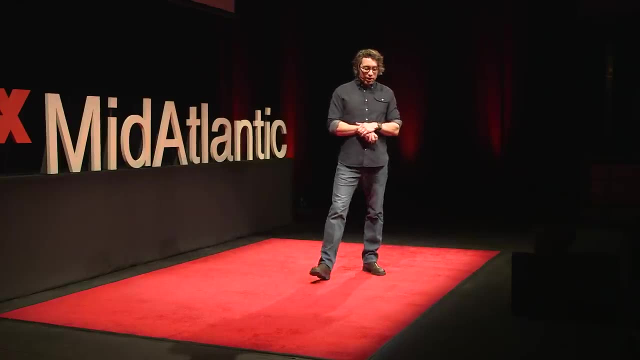 want to use way of talking about what you do and why it matters. I mean, heck, it works with two of your closest colleagues. what could go wrong when it goes out to normal people, people who don't eat and breathe and sleep? your issues all the time and you find that when this idea that made so much sense, 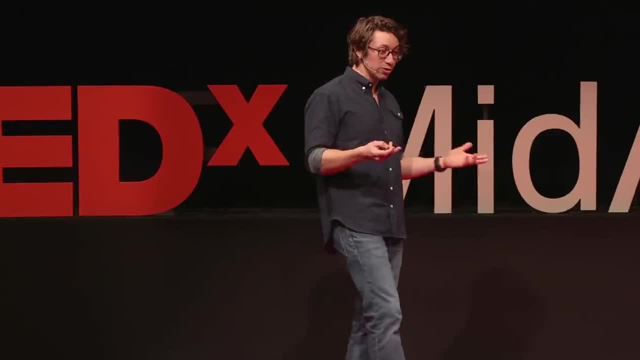 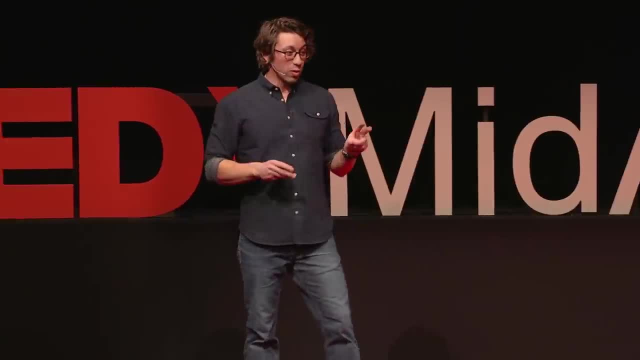 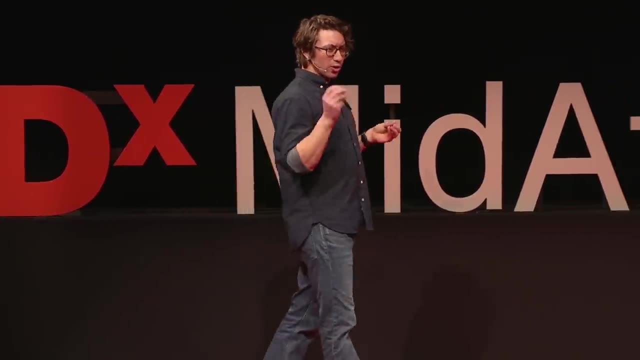 it doesn't have a grip. it doesn't have a grip, it doesn't have a grip, it doesn't in one ear and out the other. secondly- probably more unfortunately, because it happens more frequently, I think- that thing which worked and was so brilliant in your own head goes out and it has the exact opposite effect on the people. 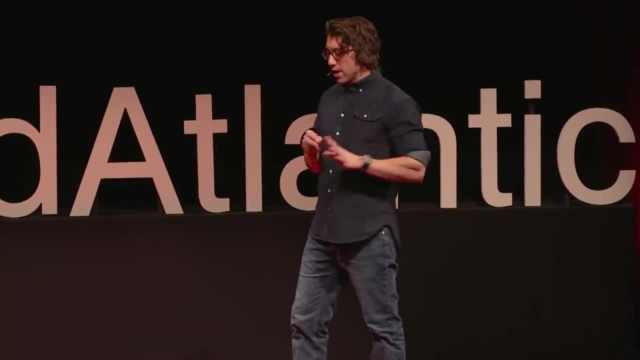 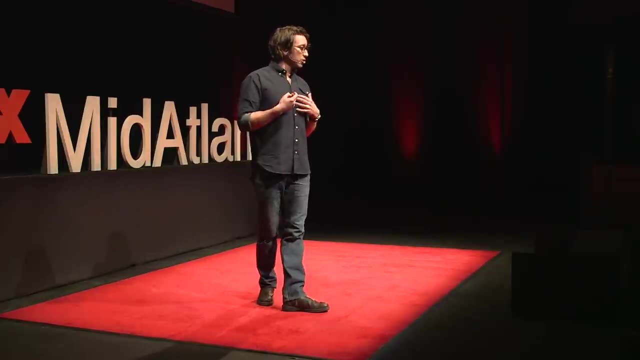 you're trying to persuade on the people you're trying to communicate with, and I'm not going to ask you to to take my word for anything today. right, I'm gonna show you evidence from the research that I do with my team that shows this, and I 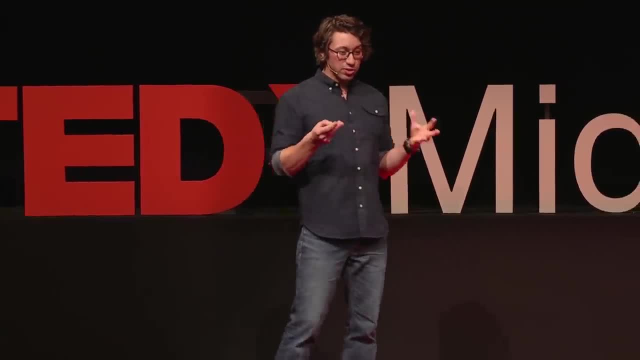 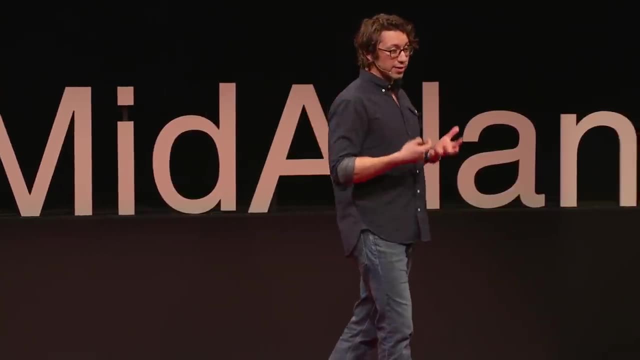 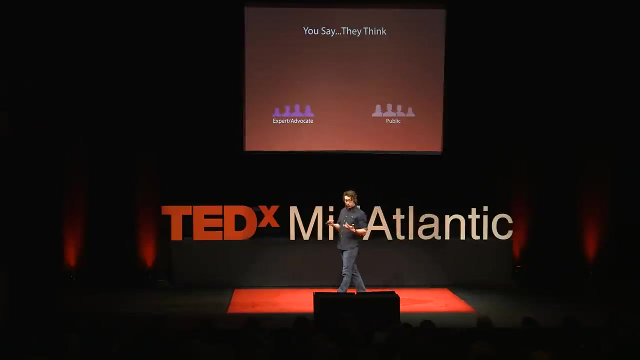 have a lot of pieces of examples of evidence of this. you say they think this loss in translation effect. I'm gonna show you one today. that comes from some work that we've done to translate the science of early childhood development, and so people who are in people are in this field, people who are developmental. 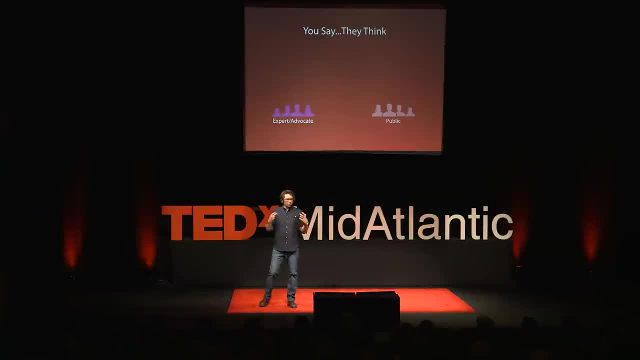 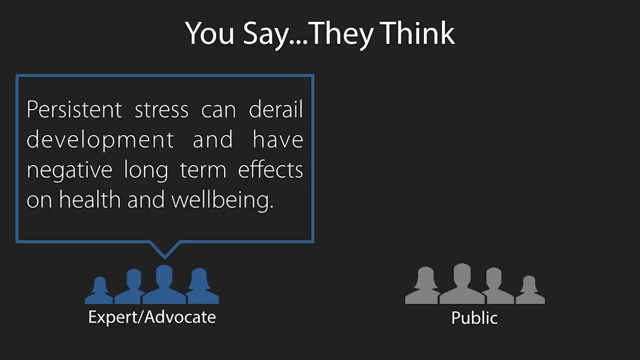 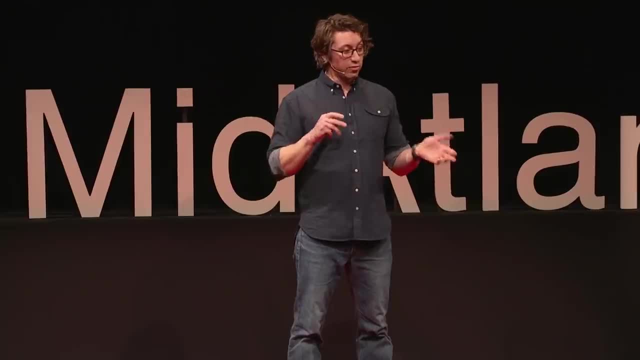 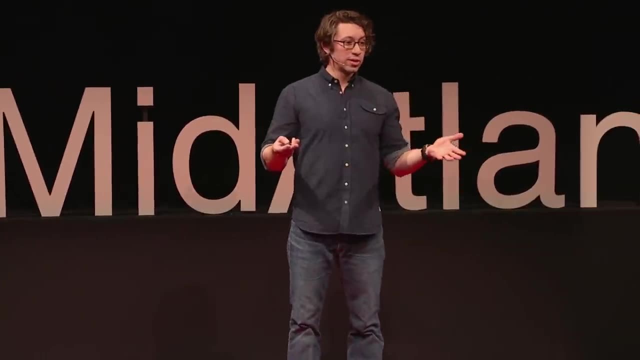 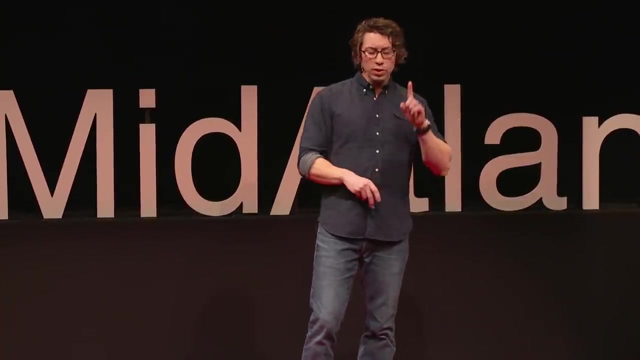 and health and well-being, and if you're a developmental scientist, you replace negative with deleterious, because that's the way you talk, and so for folks who are in this field, this is true. there is an incredibly deep body of science across a number of disciplines which supports this point. unfortunately, when 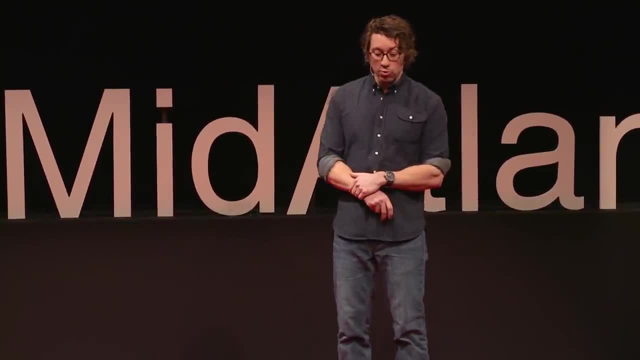 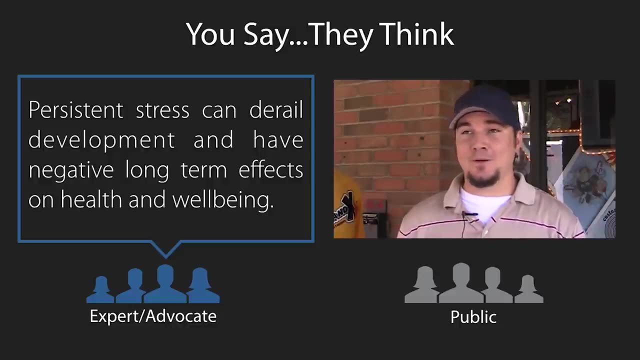 you take this idea out to normal people, to members of the general public, you get things that look and sound like this: life's hard, supposed to be hard, what, what? Life's hard, It's supposed to be hard. What doesn't kill you makes you stronger. All the bad cliches you can think of, I mean there's. 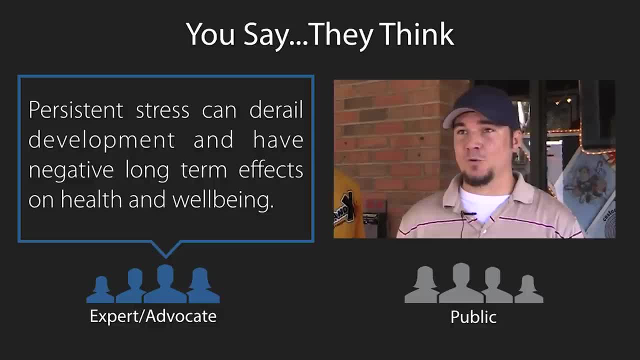 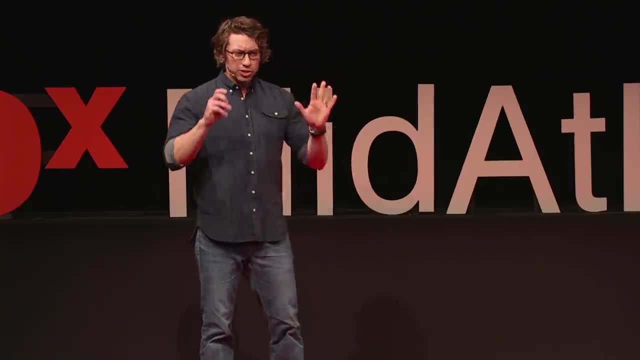 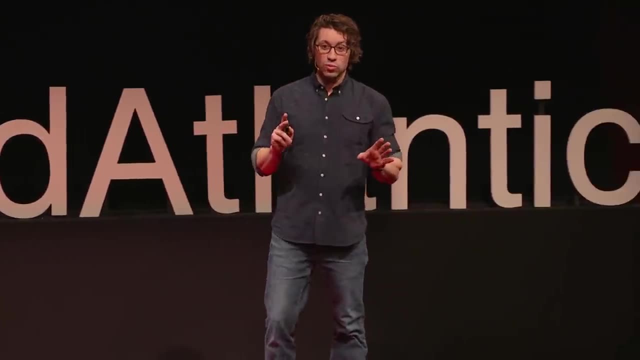 there's been people that have come from absolutely nothing to make it and whatever society's eyes deem success. So just to make it really crystal clear, that which you just heard was not the intended effect when this expert opened his or her mouth, to deliver this message, and I'm not trying to say that our 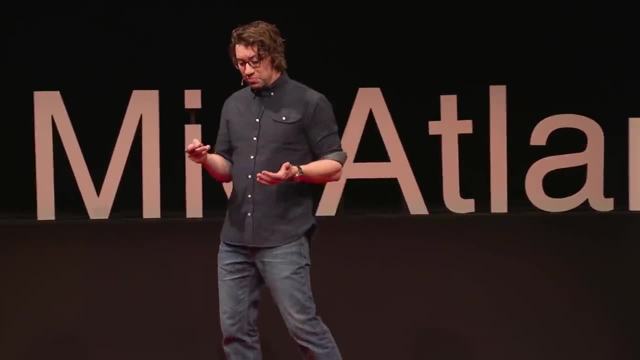 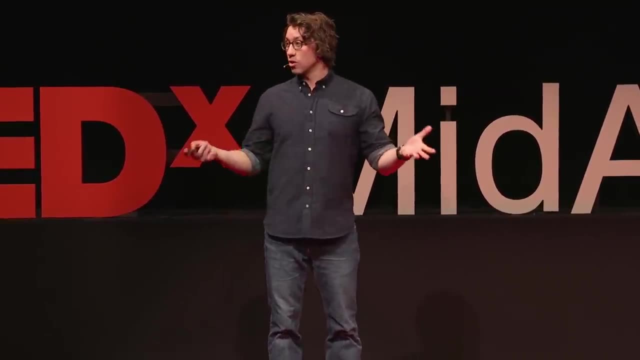 friend Nietzsche here with: what doesn't kill you, makes you stronger. smart audience. there you go is wrong or or stupid in any way, but there's clearly something that's going on here. there's clearly a difference between the, the intention and the delivery of the message and its actual perception and 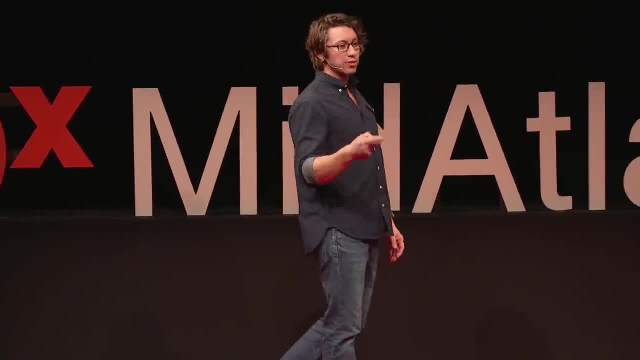 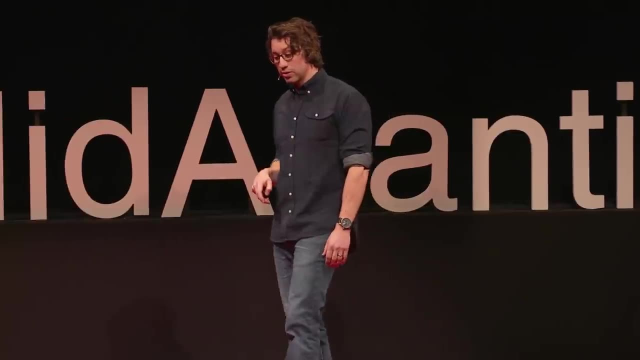 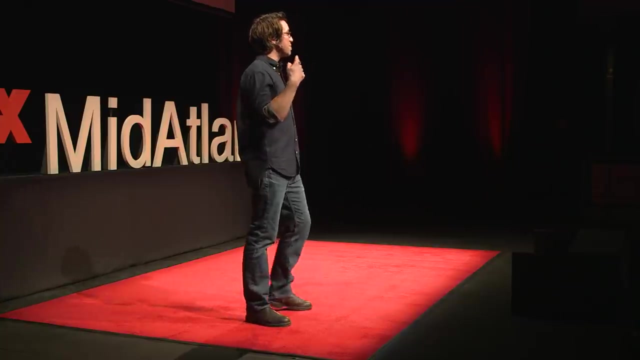 effect and you all should have a good idea as to what that is based on how I introduced myself as an anthropologist. so the thing that stands between the you say and that they think here is culture, not the external Indiana Jones artifact kind of culture, but rather culture in mind, culture as a set of shared patterns of 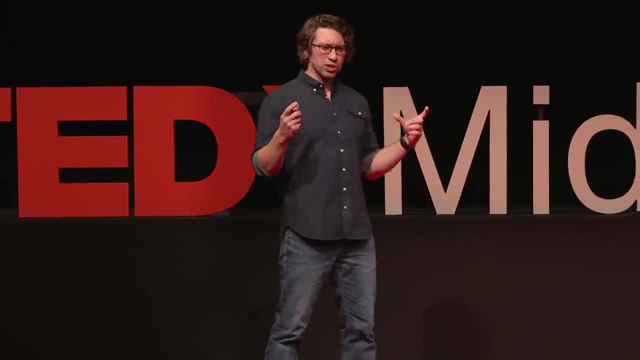 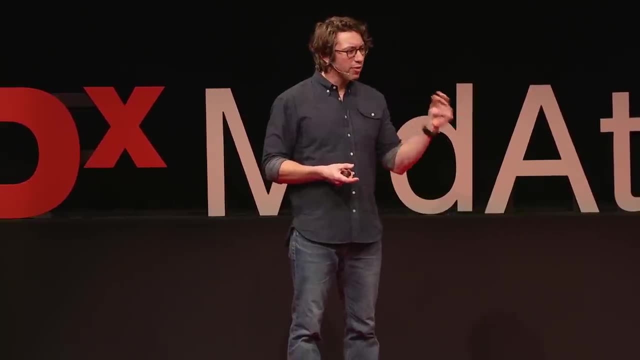 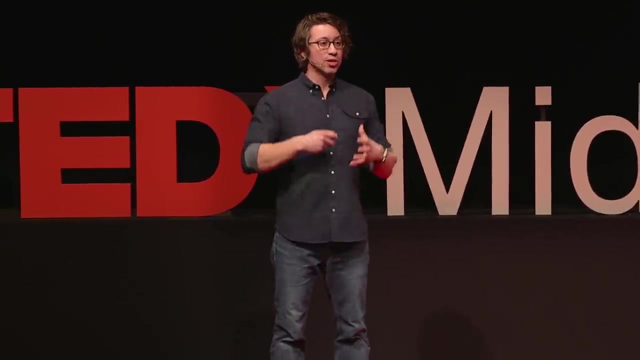 thinking as a set of shared assumptions and propositions that we have and carry around with us in our minds and use every time that we are presented with information, every time that we engage with an issue. and so what this does, this realization that culture is always mediating our meaning and complicating 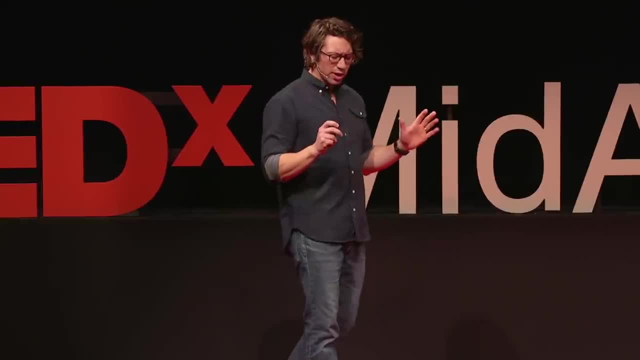 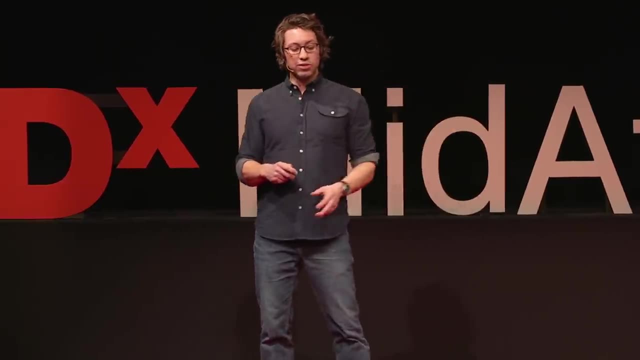 our job as communicators is it gives us. so this is both kind of one of these paradoxical things that's both utterly common sense and completely game-changing- is that this gives us a really different way of looking what at what has been the dominant way of thinking about public understanding and 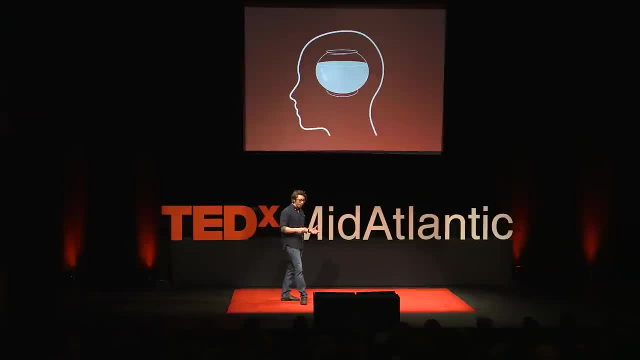 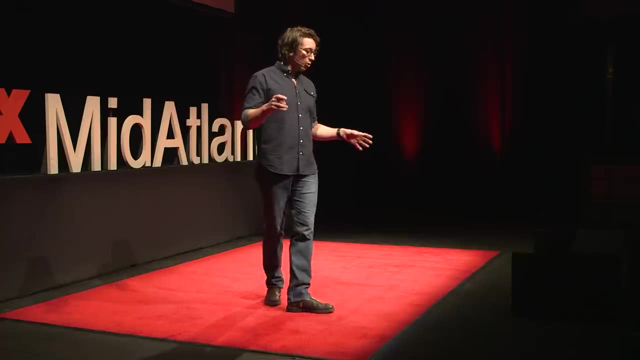 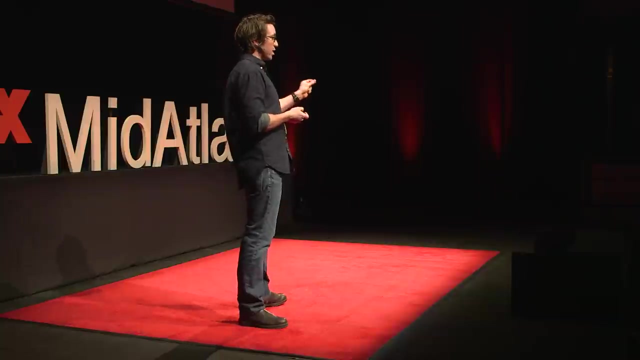 communication, and so for a long time, and still to this day, people have thought of public understanding in this way, as it empty receptacle, as a blank slate, as an empty fishbowl, and have thought that we, as communicators, can assume that we are our audiences and take the things that make so much sense to us and they're not. 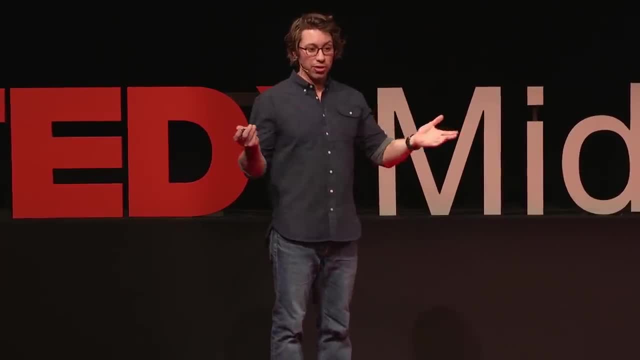 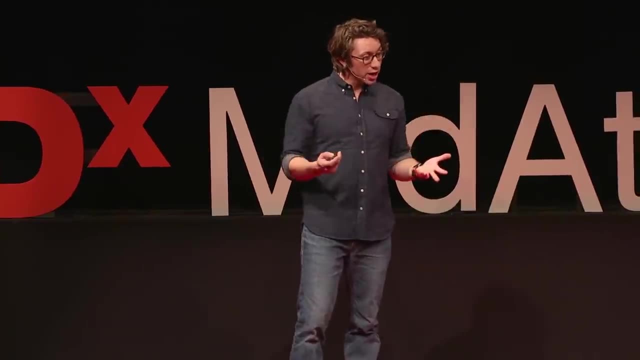 us and literally drop them into this unfettered space where they get to do their thing. and we know, based on what i've just told you about culture, that this is neither correct nor is it productive as a way to think about communications, and instead we have to understand that culture always. 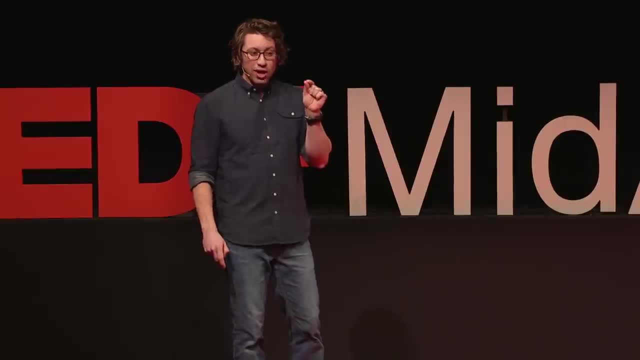 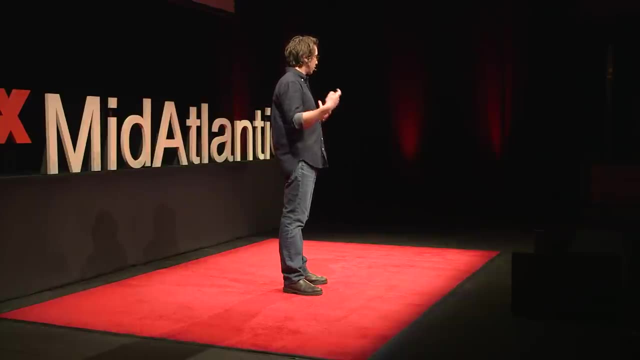 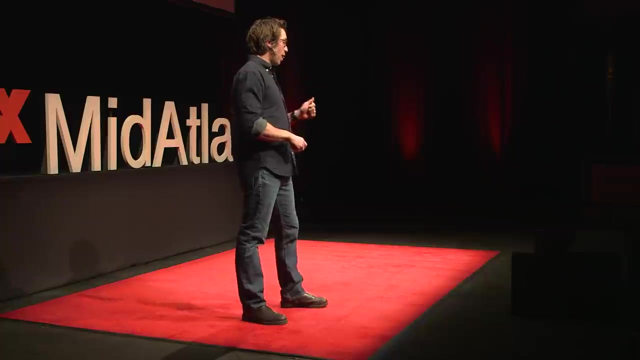 complicates our job as communicators, and if we can go a step further and understand how people use culture to think about our issues, we can be dramatically more effective in our roles as messengers, in our roles as communicators. and so the the second reason why framing matters to all. 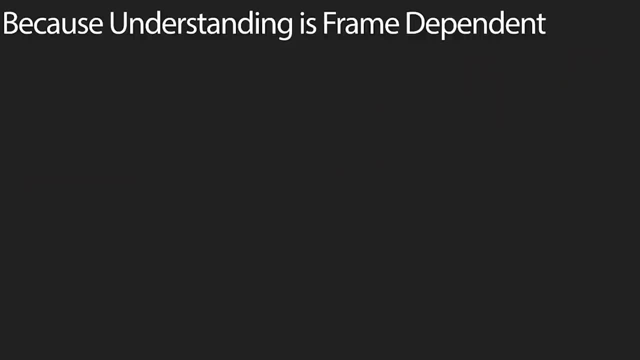 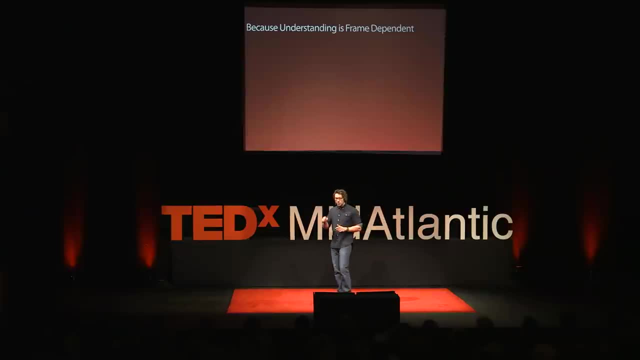 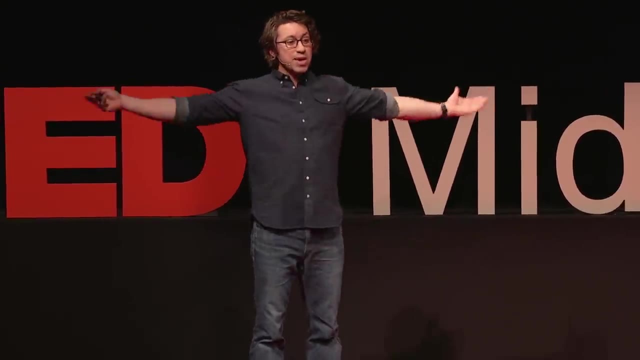 of you in this room is because understanding is frame dependent. now that's a mildly academic ease way of saying that the choices that you make as communicators matter. sometimes the little things, the pronouns that you use, the verbs that you choose. sometimes the big things, the values. 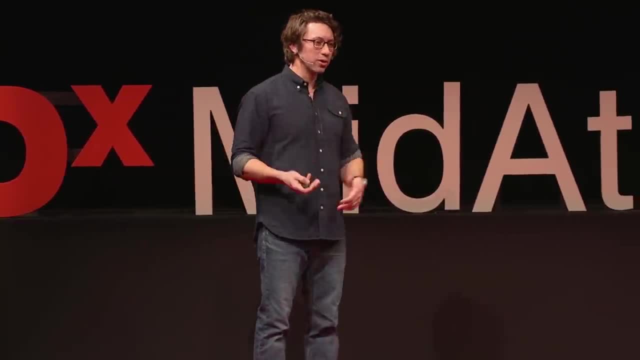 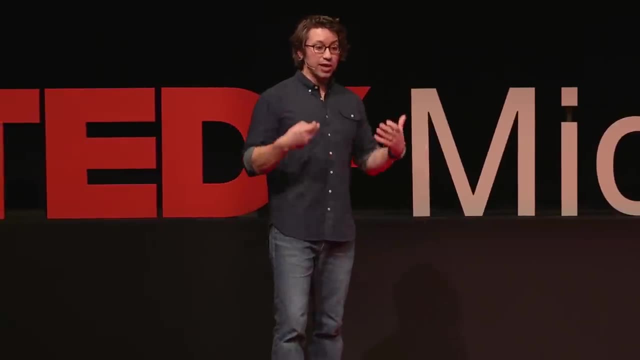 that you use to explain why your issue matters. those things matter you. those things have frequently dramatic impacts on what people are willing to do and how people are willing to act and engage on your issues and again, i don't want you to take my word for it. 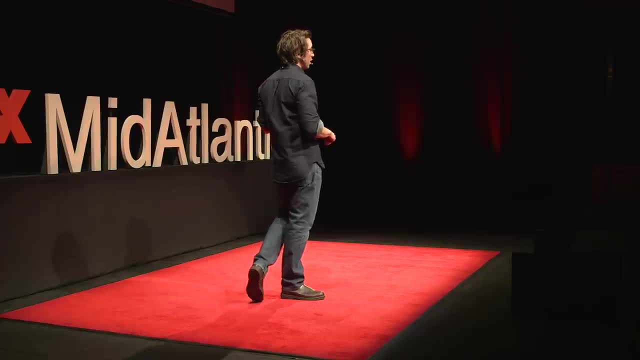 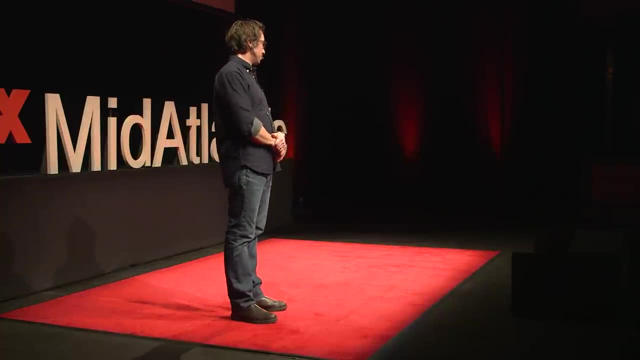 i'm going to give you a quick example that shows you that understanding is frame dependent. and this example comes not from the united states but from the canadian province of alberta. and a quick geography lesson. alberta is one of the tall, skinny ones in the middle of the country. 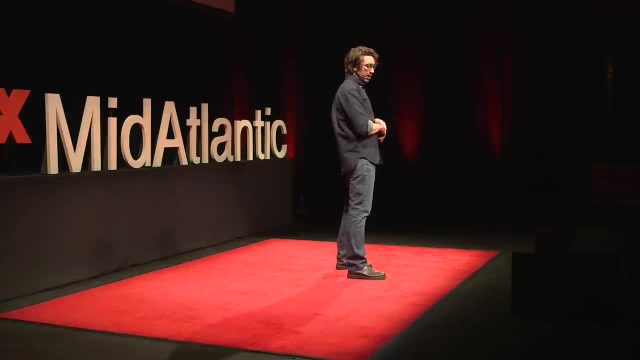 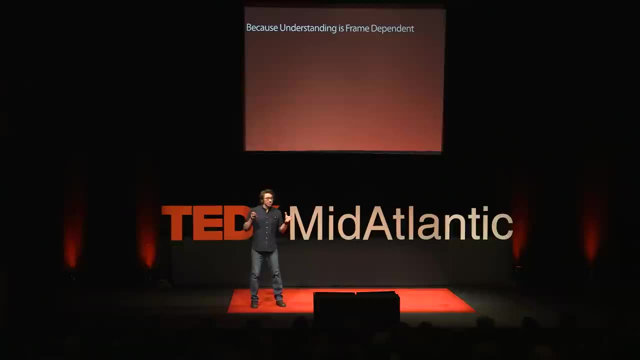 kind of all you need to know. it's very cold for this example, and so there's a group of of experts and advocates in alberta who are working to change policy and practice around addiction. they're working to take what we know from science and use it to implement better policies. 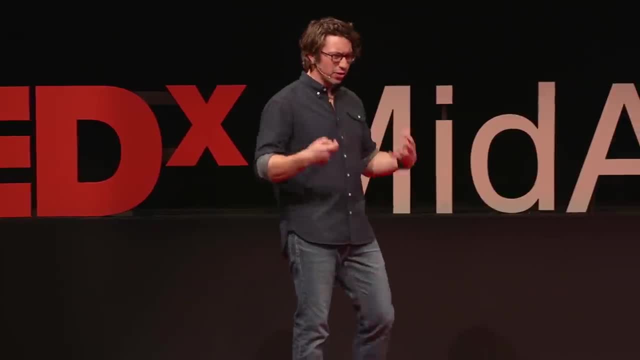 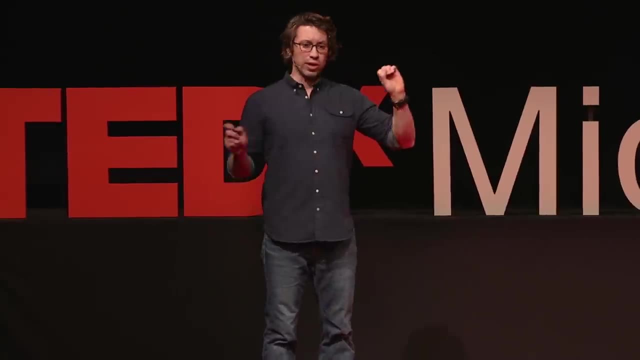 and practices around addiction in this province, and they've been having a great deal of difficulty doing this. a lot of their problem comes from the fact that there's zero support to do anything different when it comes to addiction in this province, and so they came to us. 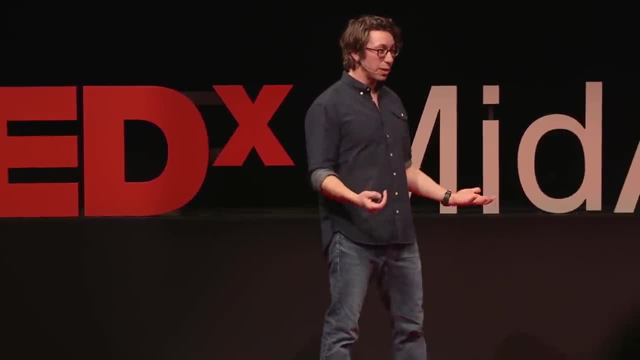 and they asked us to conduct some work to figure out how to engage members of the public more productively. and they came to us and they asked us to conduct some work to figure out how to engage members of the public more productively. and they came to us and they asked us to conduct some work. 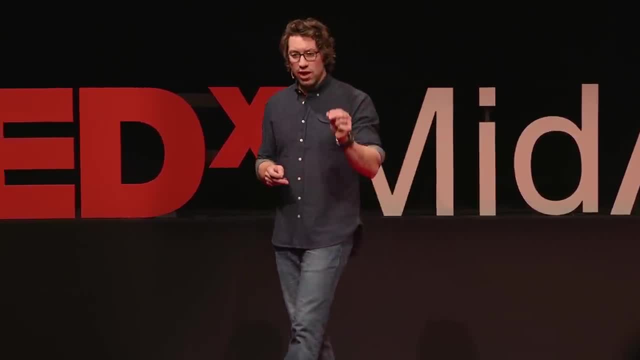 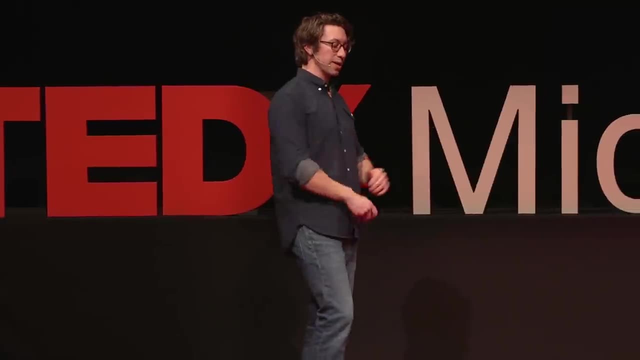 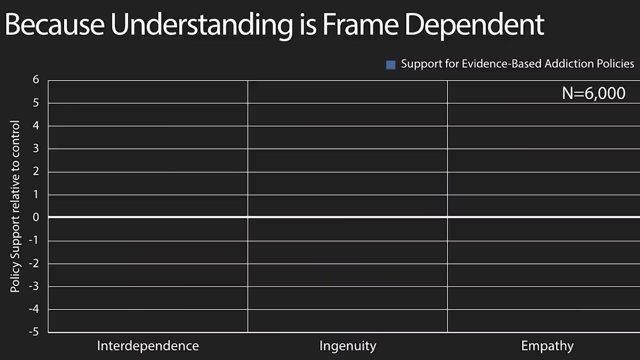 to move understanding and, specifically, to increase support for a set of evidence-based policies. and so, as good framing geeks and dweebs we do what good framing geeks and dweebs do- we ran an experiment, and in this experiment we tested three different values messages, and so you see the values messages. 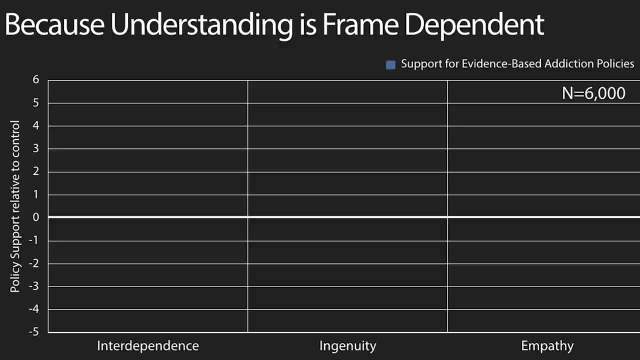 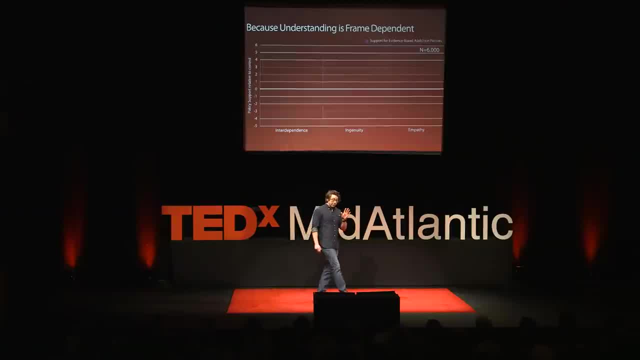 along the horizontal axis of this graph right now, and so some people. so this is a large experiment: 6 000 people, which, believe it or not, is not the entire population of alberta, it's a. it's a representative sample of six thousand people and we have a two, three hundred percent population of 6 000 people and the range of a little more is a percent of 7 000 per person. meanwhile, the average rate of oral addiction is twelve something. 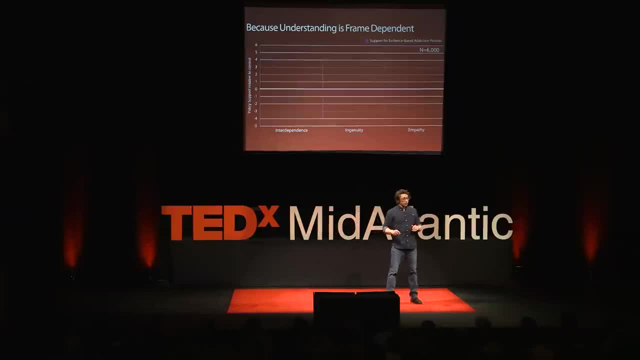 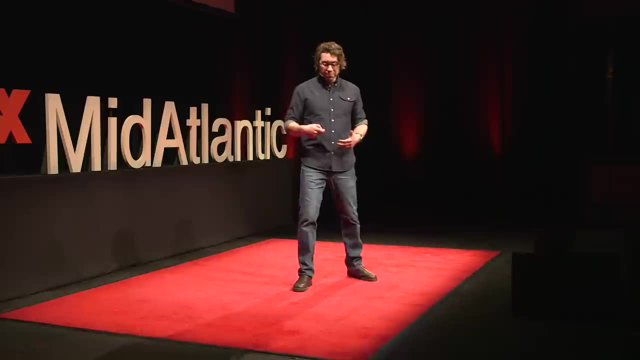 not an exhaustive sample. each of these 6,000 people is randomly assigned to one of these messages, so some folks got the value of interdependence, which, in this case, is the sense that we need to do a better job of dealing with addiction in this province, because we're all connected. what influences one of us? 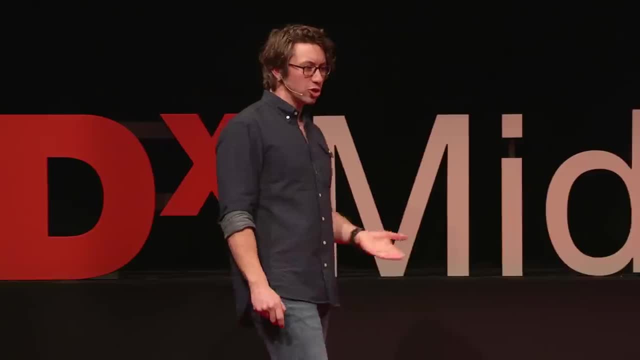 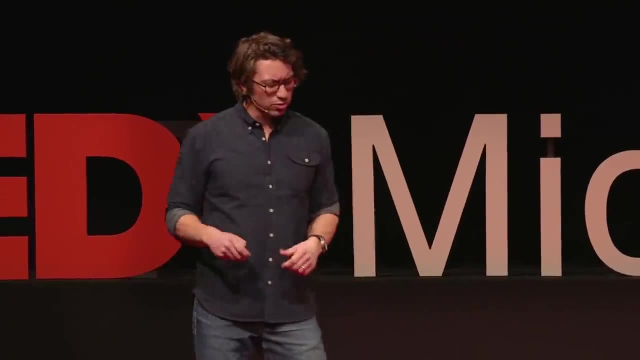 influences all of us. other folks got this value of ingenuity, which is an innovative, an innovation value that we are a province of problem solvers. you kind of swing your arm when you do this one. there's never been a problem that we haven't been able to solve with some good old Albertan grit and roll up your 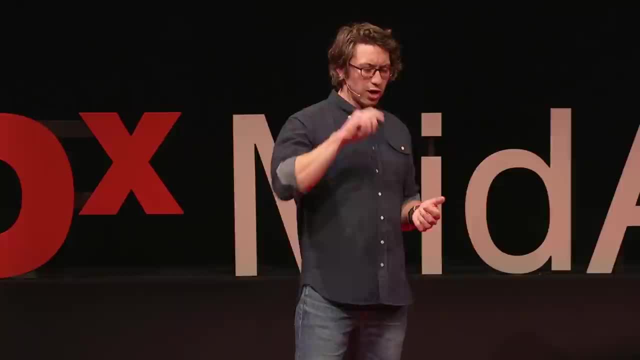 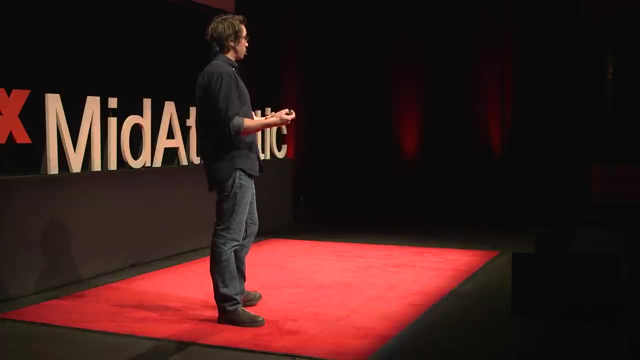 sleeves, problem solving this. that was my Albertan accent, I don't know if you caught that. that's very important and other folks, last but not least, got this value of empathy, which is the sense that we need to do a better job of dealing with addiction in this province, because people who deal with addiction are 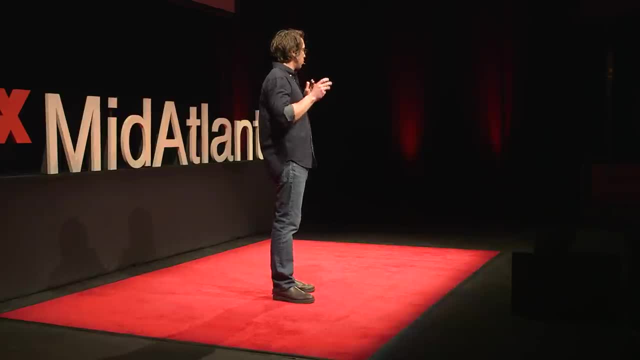 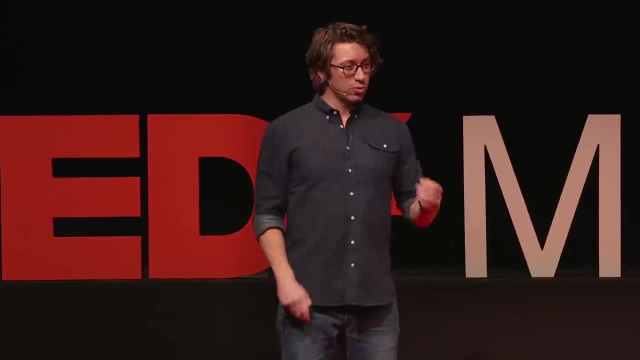 people too. they could be our mother, brother, father, sister, neighbor, whomever- and as individuals, we need to show these folks compassion. so what you're gonna see on this next click is what I think are three beautiful blue bars will appear on the screen, and what those blue bars are going to show. 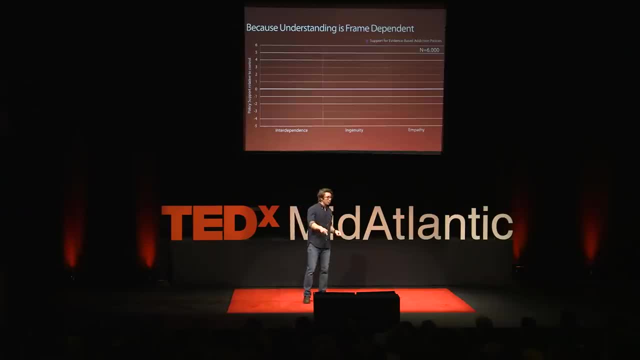 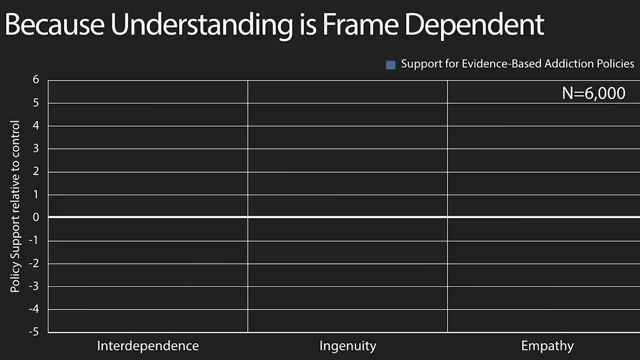 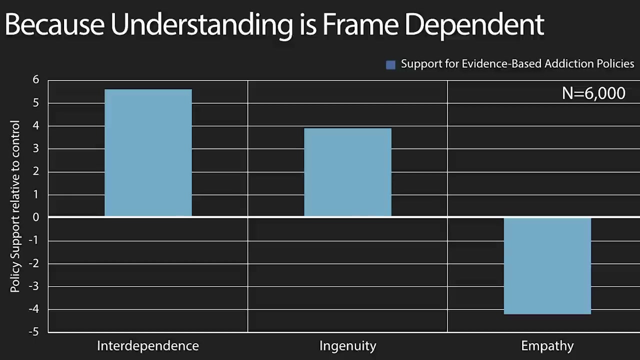 you is the extent, the degree to which hearing these different values changes people's support for these evidence-based policies. so can anyone do a good drumroll? please play along. thank you, thank you, thank you. so you should see three blue bars and notice two things. so first of all, two of these. 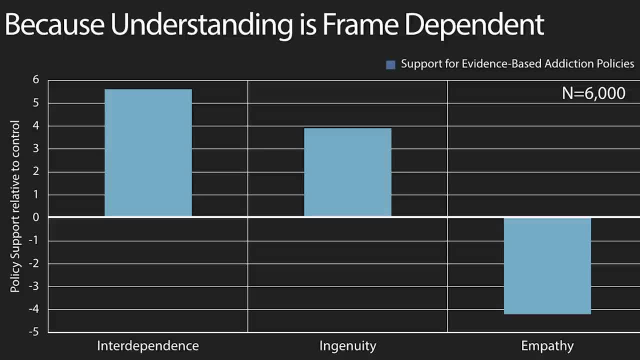 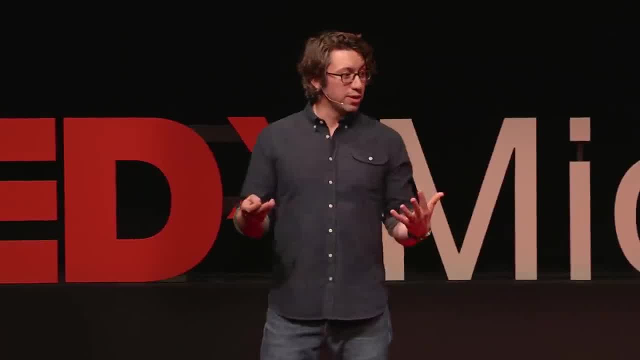 values, interdependence and ingenuity make people, to a statistically significant degree, more supportive of the values that we're dealing with, and the second thing is that we're dealing with a very significant number of people who are not necessarily the most supportive of these evidence-based policies. that is good news. when we run these experiments and when we get 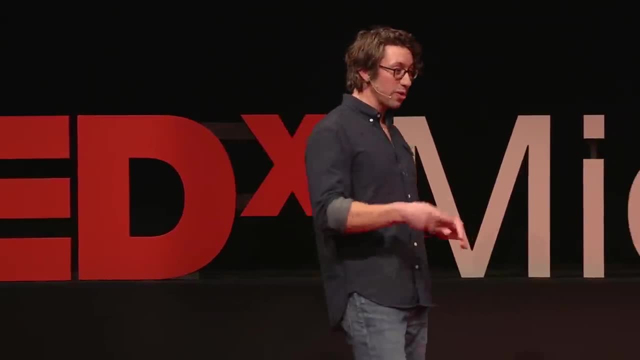 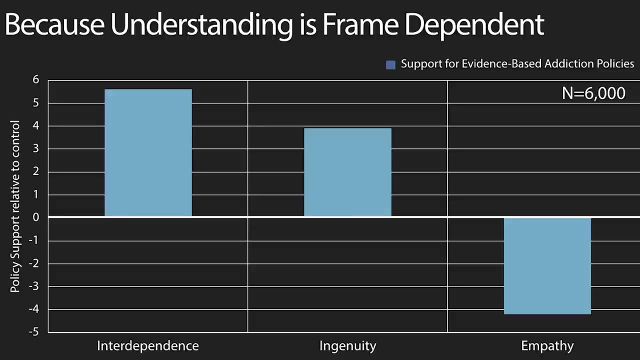 results like that. we stand up, we do a little framing dance- not gonna do it right now, don't worry- we sit back down and we look towards the right-hand side of the screen. the value of empathy is actually depressing people's support for these policies right now. the kicker is that in a subsequent piece of analysis, 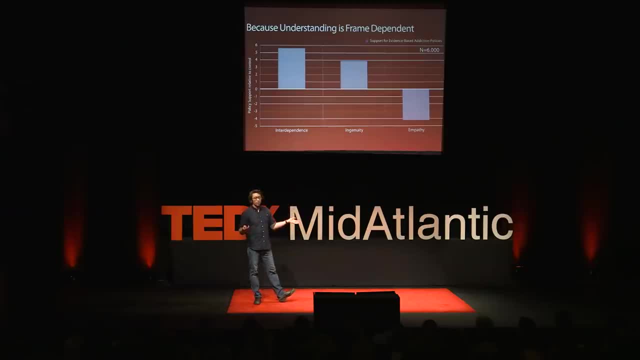 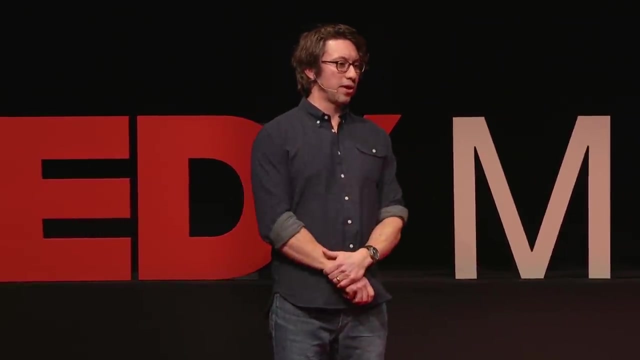 where we looked at all of the fields- external facing materials, guess which? and we looked at the last segment that was reported up here. it was a 2.3 percent out of 90 percent of the time- empathy, thank you, not a rhetorical question. and so what this field has been doing for a very long time is endorsing 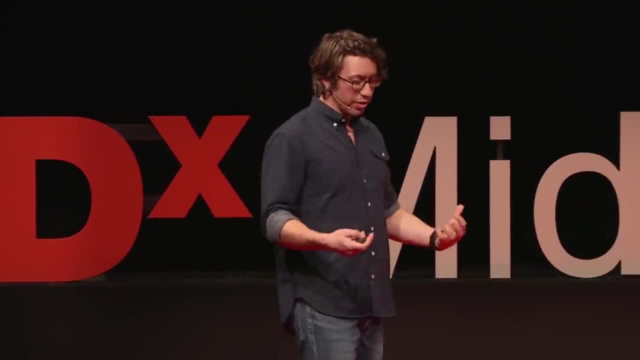 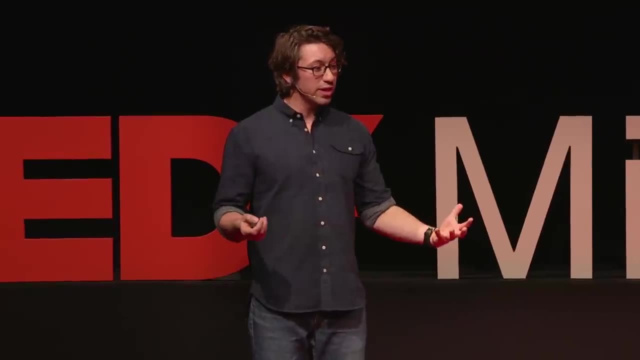 a value which actually drives support down for the very policies that they're advocating. so this, this example, does two things. it clearly shows you that framing that understanding is frame dependent and frames matter. it also shows you that these questions- we know which values to use, how to communicate our 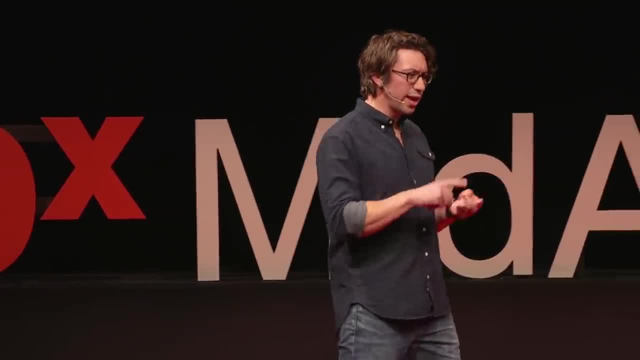 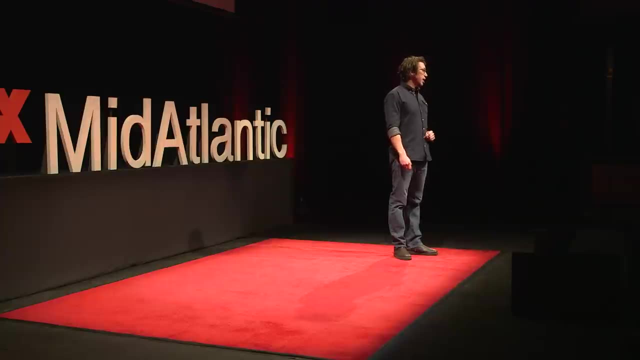 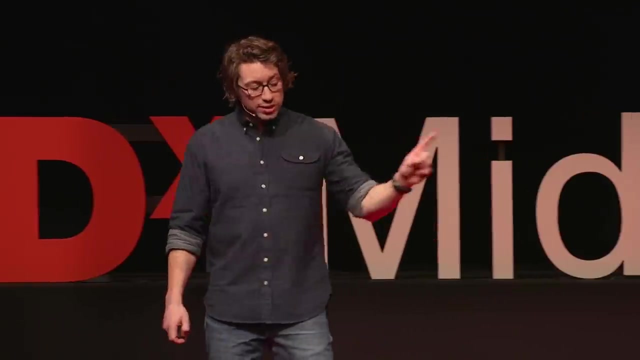 And so I think it's pretty cool that frames are able to move people's understanding and their policy support. But what about more intrinsic subconscious thinking? What about implicit bias? Can frames make people less subconsciously biased against particular groups of people? So we set out to answer this question through a project on reframing aging in which we were 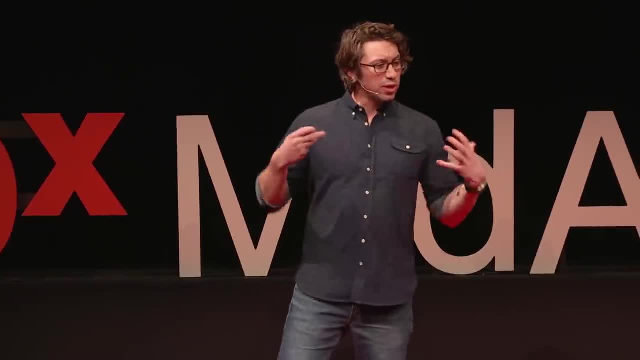 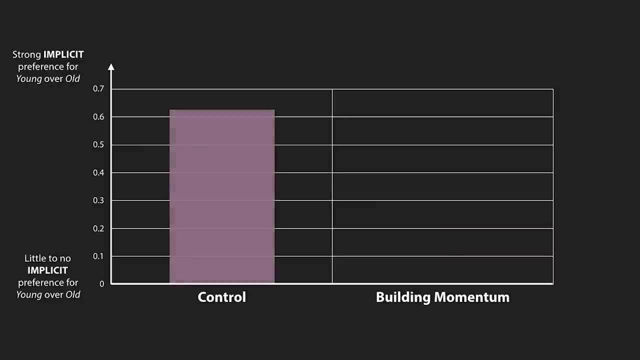 specifically interested in, can frames make people less implicitly biased against older adults? And we found two things. So, first of all, Americans do not like older people. Older Americans don't like older people. High degree of implicit bias, and it's a level of implicit bias that parallels other biases.